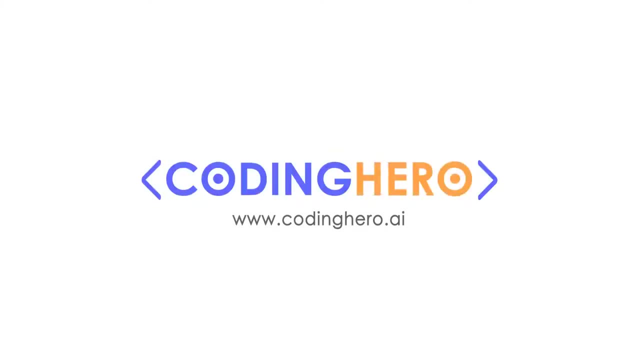 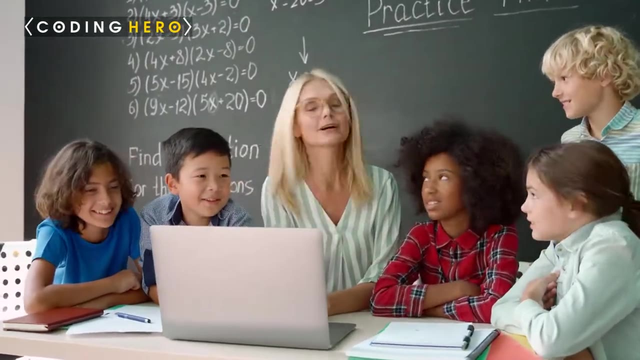 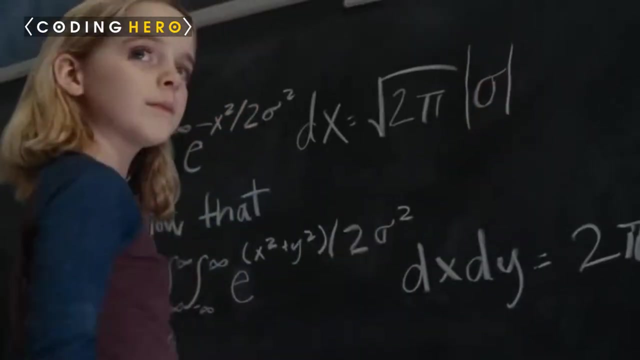 Many people believe that math is just the use of complicated formulae and calculations, which is never applied in real life, But the reality is, math is a universal language that is applied in almost every aspect of life, from playing games to playing music. These are the areas where we are constantly using math. 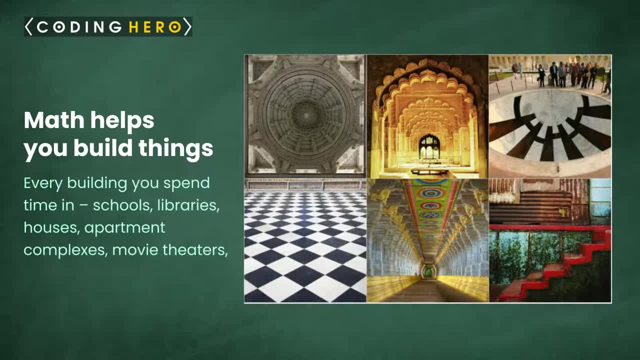 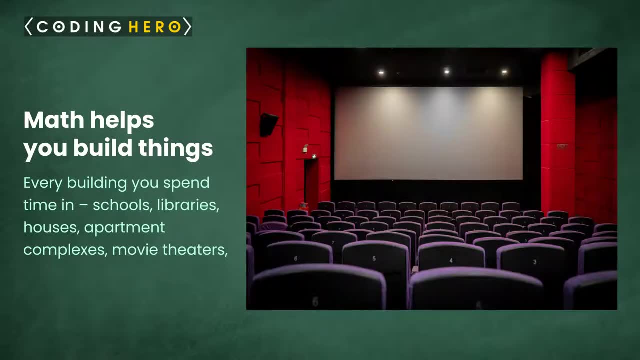 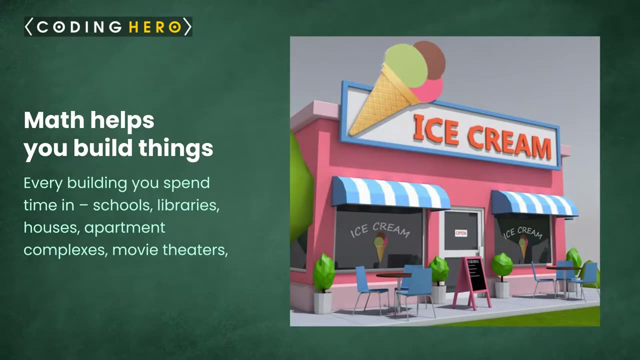 in our daily life. Math helps you build things. Every building you spend time in schools, libraries, houses, apartment complexes, movie theaters and even your favorite ice cream shop is the product of mathematical principles applied to design and construction. Math helps you keep fit, Although maintaining fitness is. 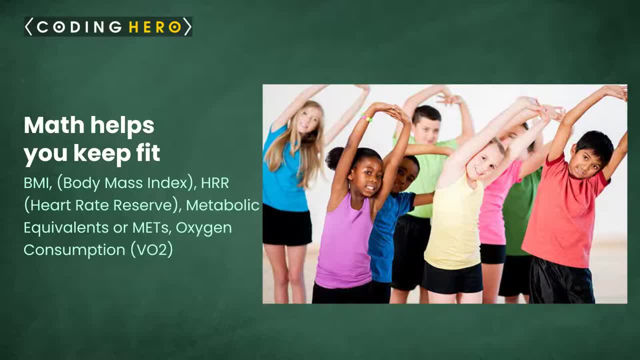 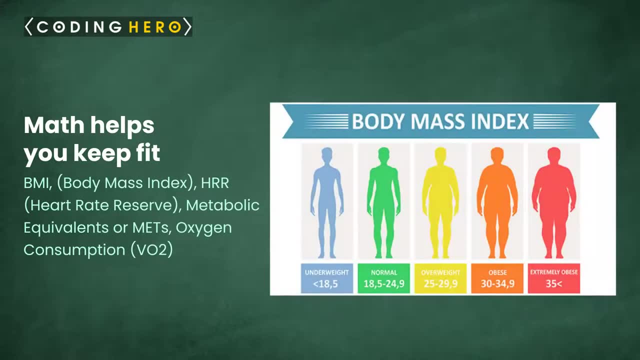 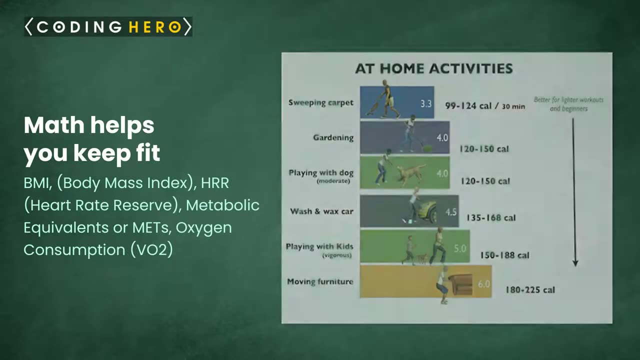 not commonly thought of as quantitative activity, but math is incorporated in all areas of exercise. Look at these examples, These terms used in the fitness world- BMI, body mass index, HRR, heart rate reserve, metabolic equivalence of METS, oxygen consumption, VO2, etc. would not be. 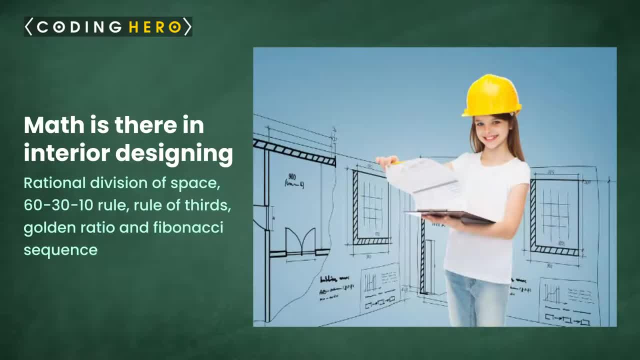 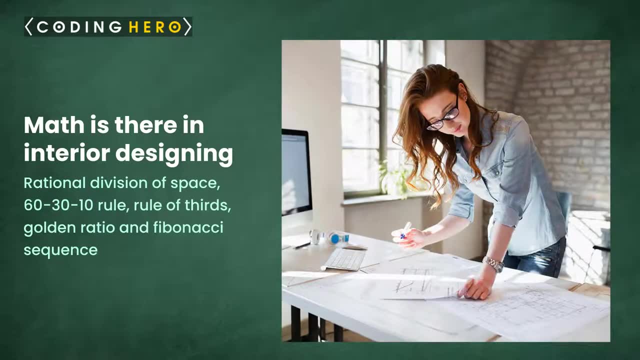 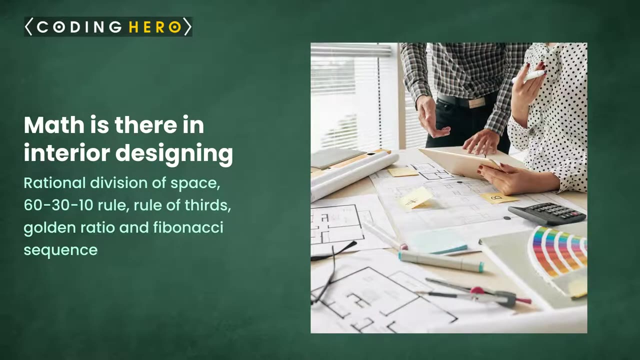 there without math. Math is there in interior designing. A lot of mathematical concepts, calculations, budgets, estimations, targets etc. are followed in this field. Some of the widely used principles of math used in interior designing are rational division of space, 60-30-10 rule, rule of thirds, golden ratio and the 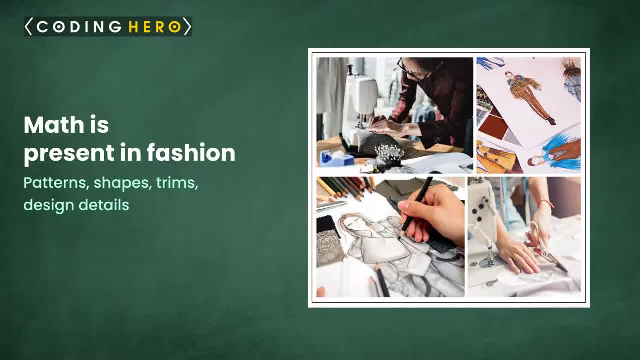 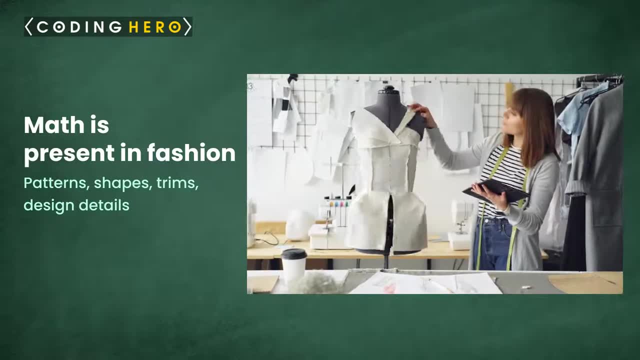 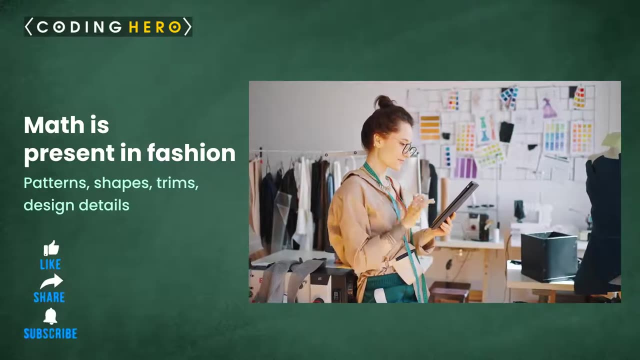 Fibonacci sequence. Math is present in fashion. The fashion industry is not just about clothing shopping and models. It has a lot of math incorporated in the day-to-day operations. Fashion designers totally depend on math for creating patterns, shapes, trims, design details and, in fact, every aspect of the apparel. 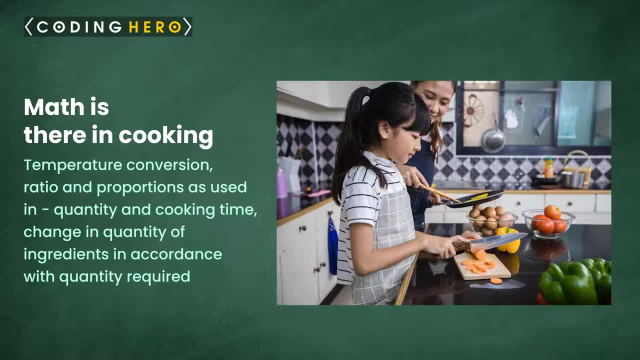 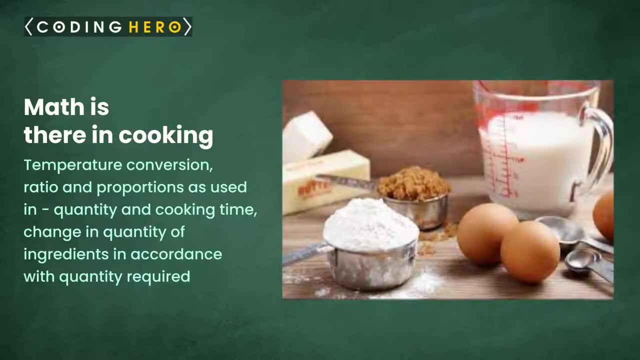 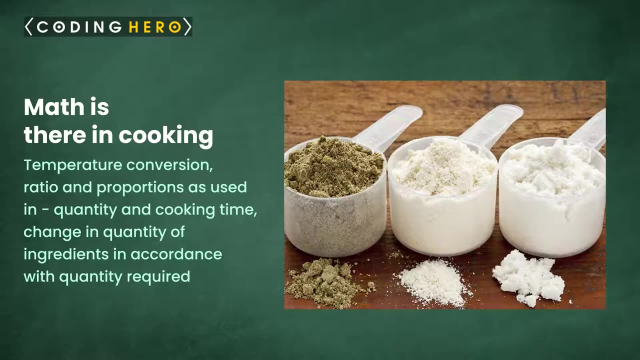 design created. Math is there in cooking. Maths is in every kitchen, on every recipe card and at each holiday gathering. Some of the concepts of math used in cooking are temperature, conversion, ratio and proportions as used in quantity and cooking time change in. 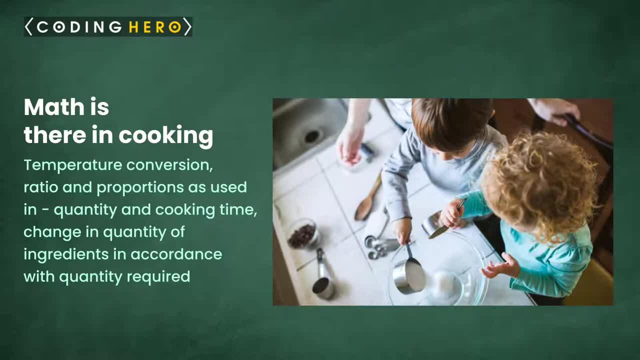 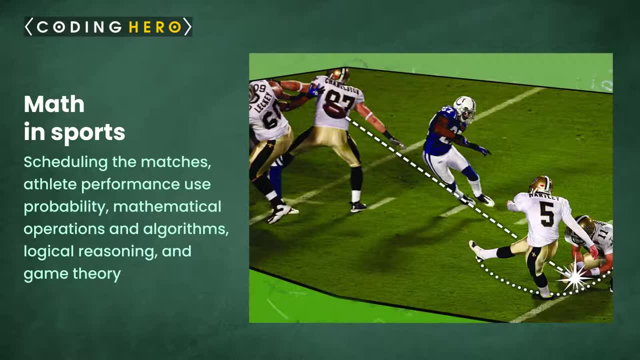 quantity of ingredients in accordance with quantity required, etc. Math in sports. In recent years, with the development of technology, math has played a more and more important role in sport, From amateur athletics to lifestyle and training in other agricultural fields. math has sharp thumbs. because these other areas be important. 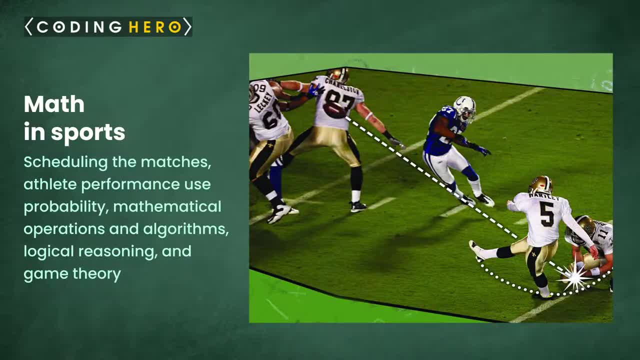 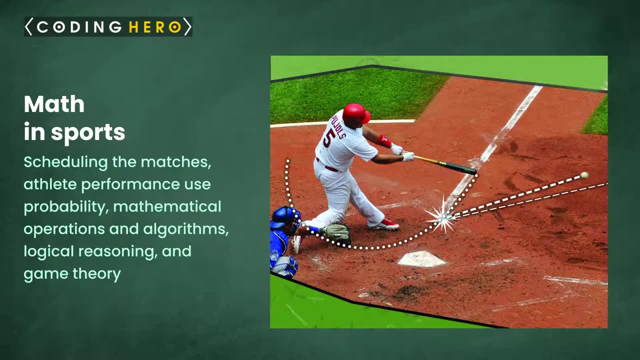 to our life if we like to be creative. It does meet more and more requirements our training to high-level sporting prowess. technology using math is used to give athletics feedback. Scheduling the matches in a tournament involves a lot of math. Some of the most frequently used concepts of math in sports are: 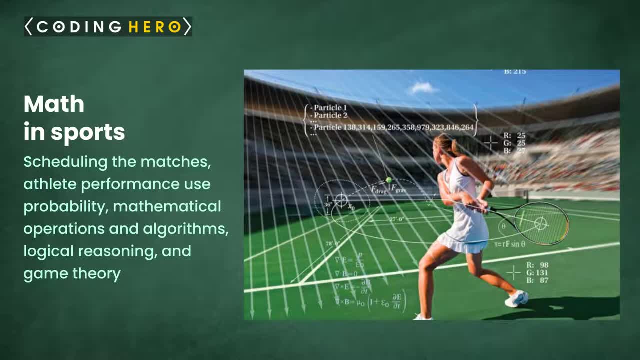 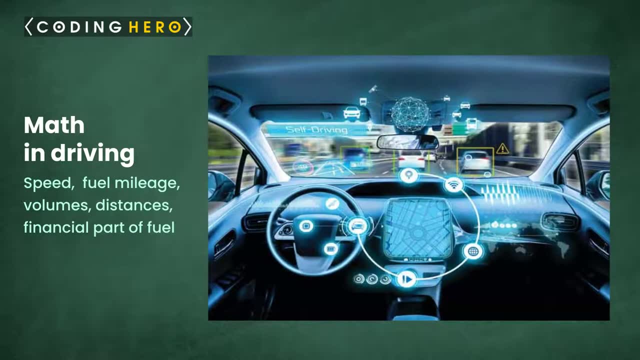 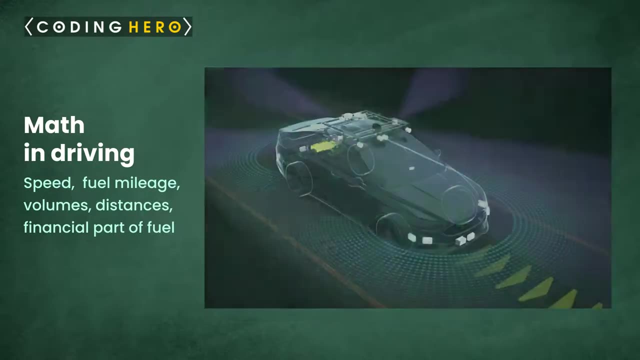 probability, mathematical operations and algorithms, logical reasoning and game theory. Math in driving: When driving, math is being utilized both in general understanding and actual use. You use math to make calculations and adjustments as you drive. You need to understand math skills to know how your 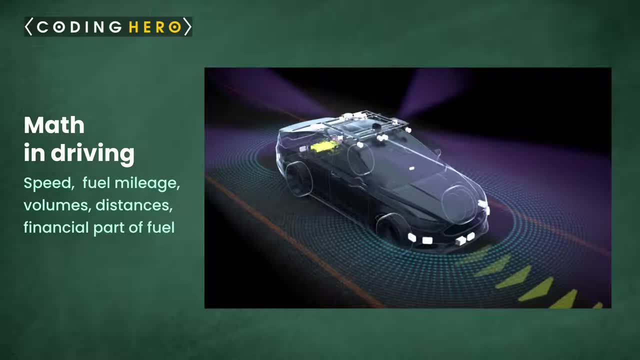 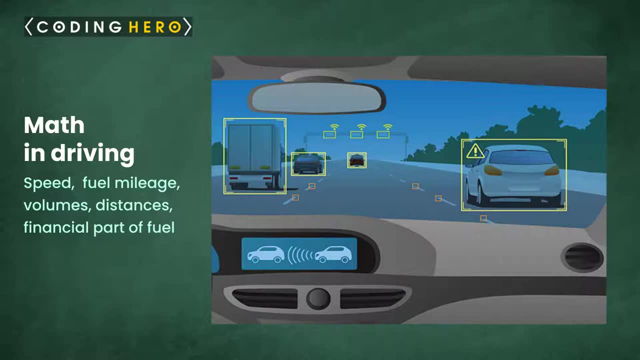 vehicle is operating and how the environment is changing around you as you drive. The most visual aspect of math while driving is speed. Another example of math would be the fuel. Math helps in understanding the concept of fuel mileage, volumes, distances and even the financial part of fuel. 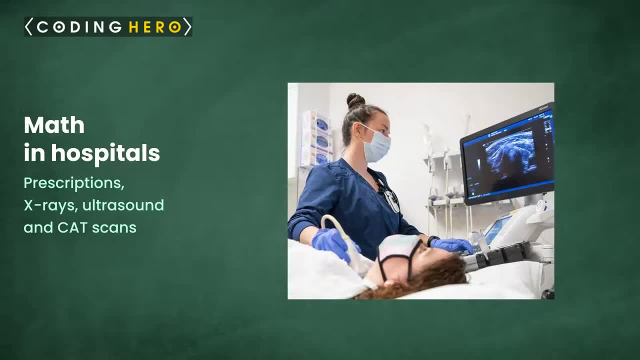 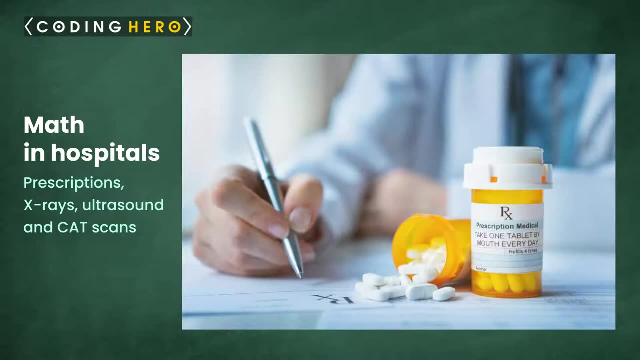 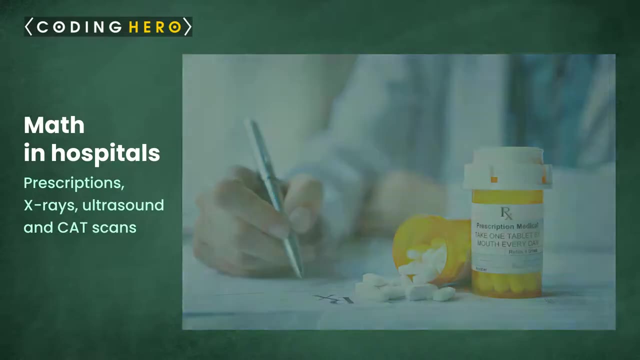 Math in hospitals. Both doctors and nurses use math every day while providing health care for people around the world. They use math when they write prescription or administer medication. Medical professionals use math when drawing up statistical graphs of epidemics or success rates of treatments. 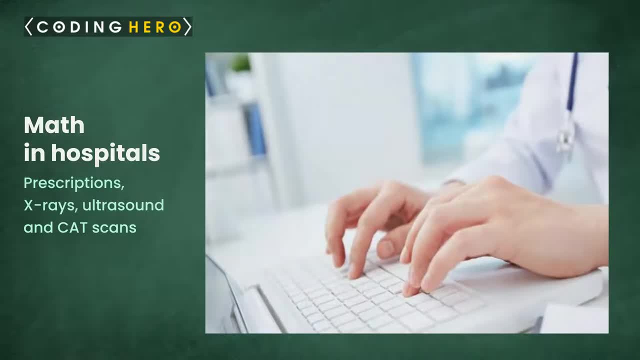 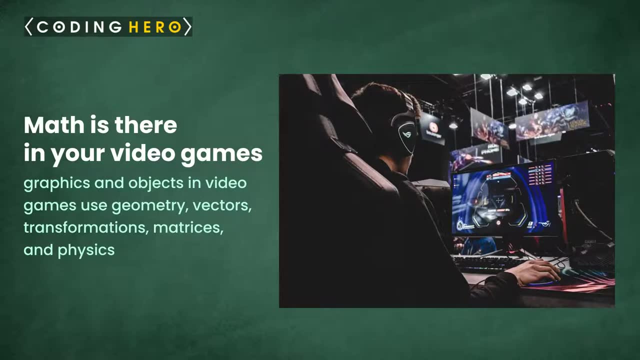 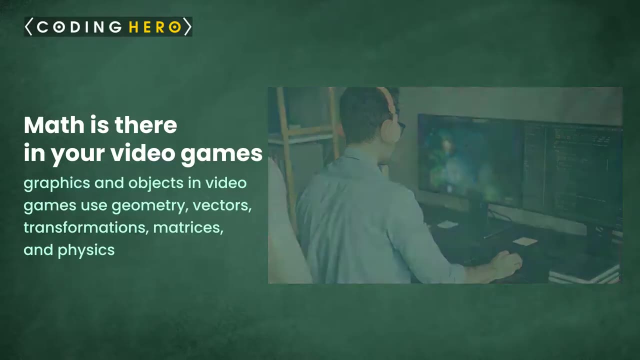 Math applies to X-rays, ultrasound and CAT scans. Math is there in your video games. There are many mathematical principles behind the creation of computer games, including geometry, vectors, transformations, matrices and physics. Many games nowadays take place in the 3D virtual world. 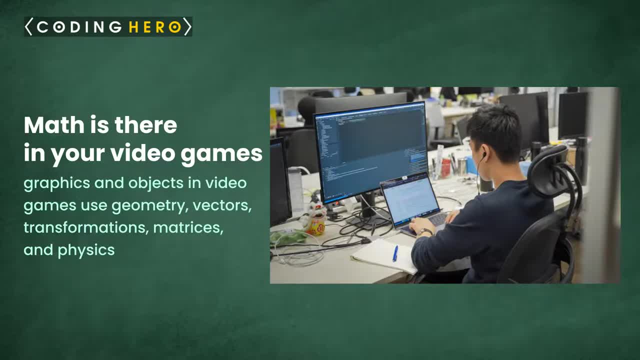 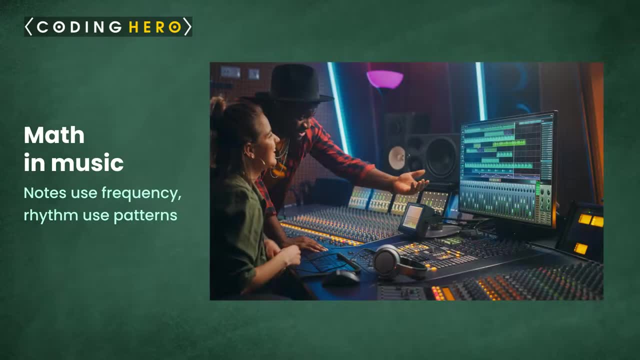 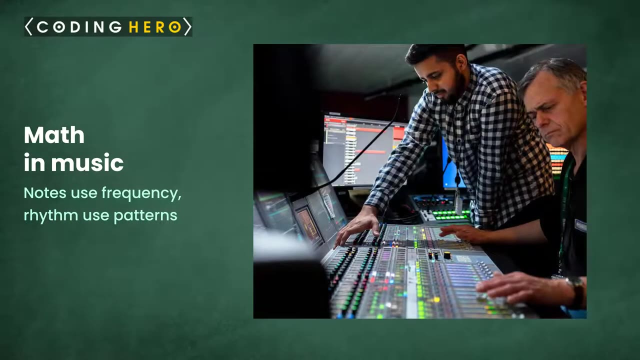 Objects and characters are created from a set of 3D points. Math in Music, Numbers, tell us a lot of information about a piece of music. Music is divided into sections called measures, and each measure has equal amounts of beats. Two important concepts of math used in music are: frequency: the shorter. the string, the higher. 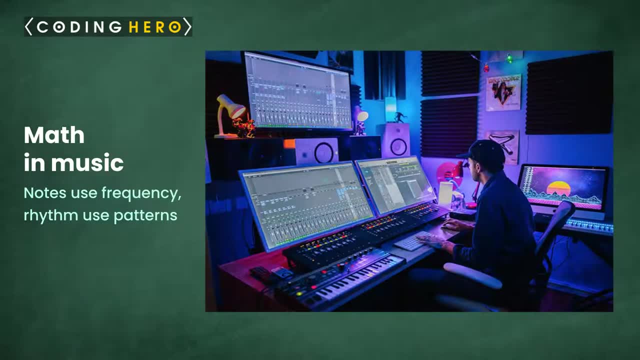 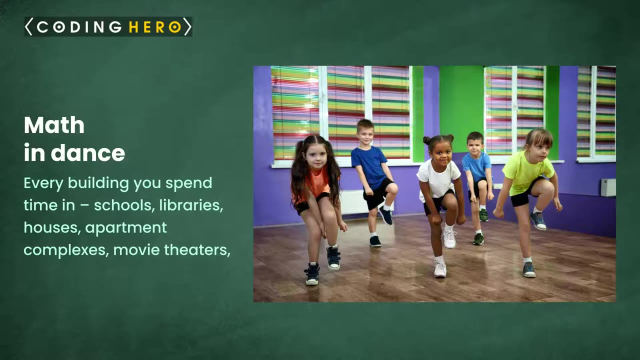 the pitch and the longer the string, the lower the pitch and pattern. Music has repeating choruses and sections of songs, and math patterns are used to explain and predict the unknown Math. in Dance, To some, math is generally seen as a bunch of numbers and formulae, which is considered to be a near polar opposite of dance.